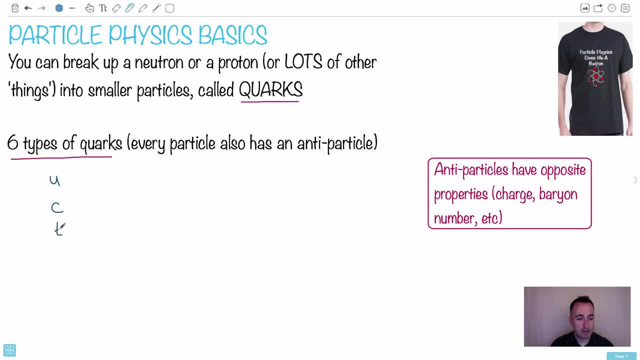 there's the up. well, we'll write them like this: U, C, T and D, S, B, And then I'll name them all. So U is called up. Now these names are kind of arbitrary, although some of them are kind of. 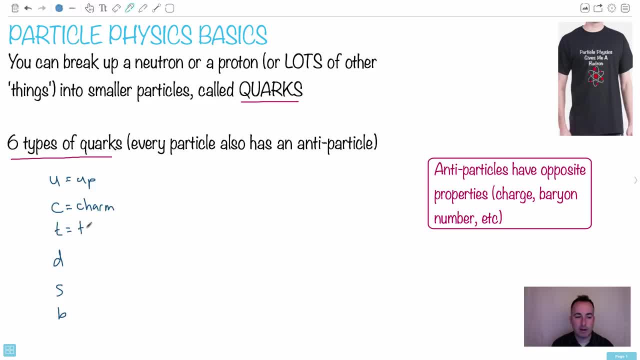 paired up for different reasons, which we don't quite need for IB. But U is up, C is called charm, T is top, D is down. We have S, which is called strange, which I think is a fun one, And then we've got B, which is bottom. So this is what you need. So you've got up charm top. 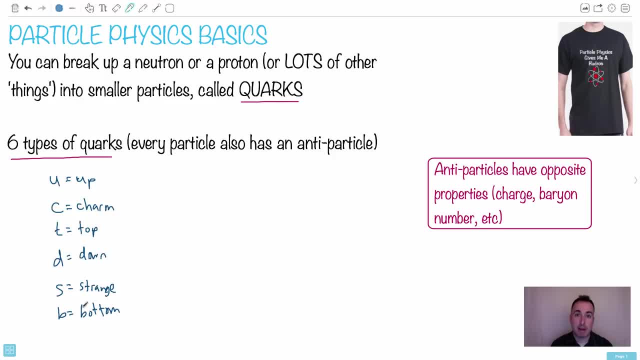 down, strange, and bottom quark. Those are those six basic quarks. However, each of the quarks has its anti-particle, Now anti-particles. they have opposite properties. So, for example, charge, baryon number- we're going to talk about lepton number and strangeness- So they all have opposite. 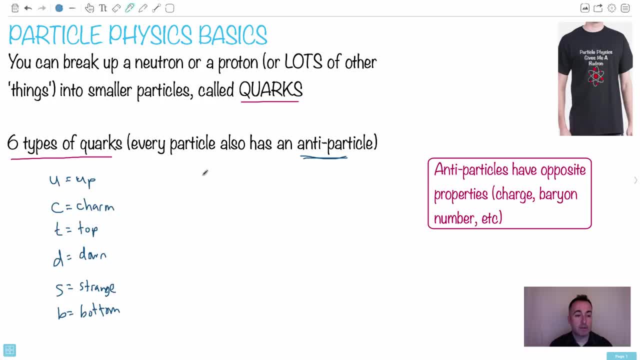 particles, opposite properties. So for example, there exists a baryon number and there are two, something called the. well, we'll write them down again. so uct, dsb. except for each of them we put a line on the top, so that tells us it's the anti particle. so if you have a up, you have something. 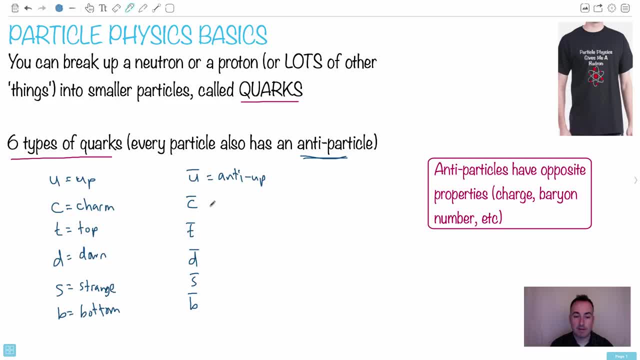 called the anti up, and if you have a charm, this is called the anti charm. i hope you get the idea here. this is anti top, uh, anti bottom, and so on. so i think this is- uh, this is actually really interesting because you have these anti particles and an anti particle is really strange because if 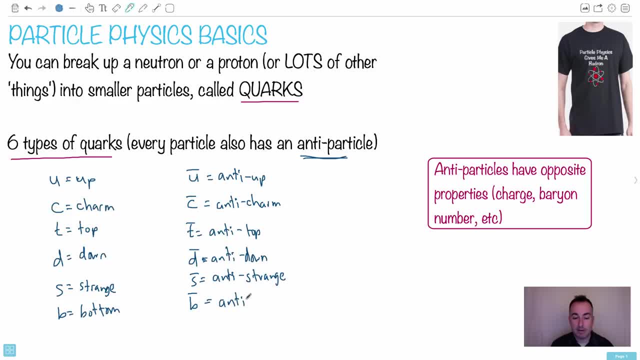 if a particle meets its anti particle, something very, very special happens. okay, i'll just make sure i spelled this right. so anti charm, top down, because when i'm talking maybe there's a big chance i made a mistake. okay, good, so, for example, if you have a particle, that's anti charm. 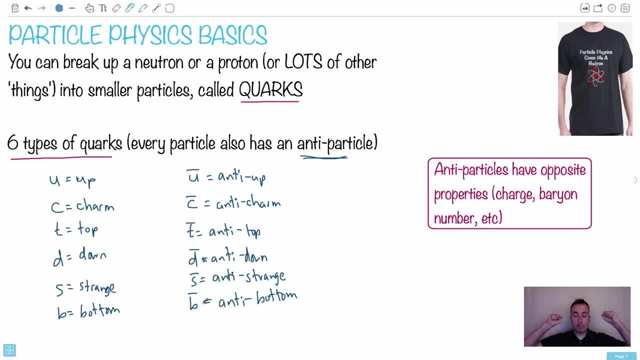 like an anti-up running into an up. So a particle and an antiparticle. If they meet and collide they actually annihilate. They make well photons basically. So this is really interesting. For example, an electron and its antiparticle. 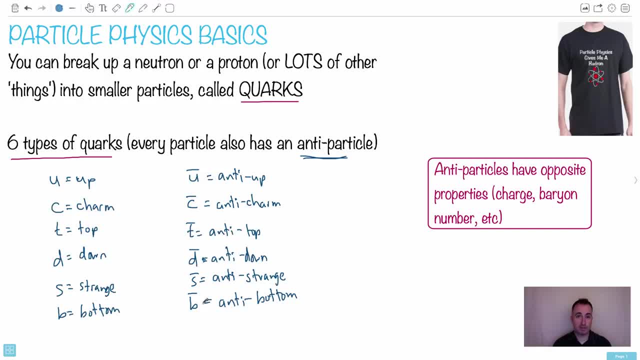 are called a positron. That was something from the nuclear physics part. If an electron and its positron, you know they're opposite particles. If they meet they disappear. We call it annihilation. They make photons. We're going to learn with the Feynman diagram. 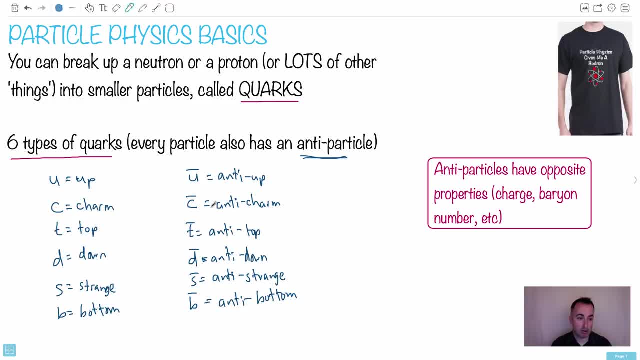 what that looks like. So basically, you just have to keep in mind there's particles and there's antiparticles. These are quarks. Now, the thing I think that causes a lot of students problems is this idea about this sort of the structure of this. 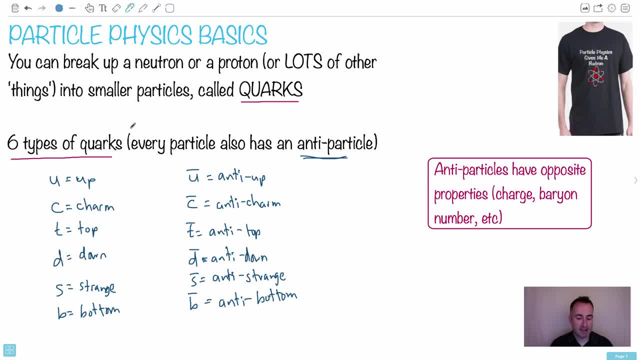 like how they're organized and how they're structured. I think a lot of textbooks just write a bunch of sentences. They'll say you can make a lot of particles out of quarks. You can say hadrons are made of quarks. 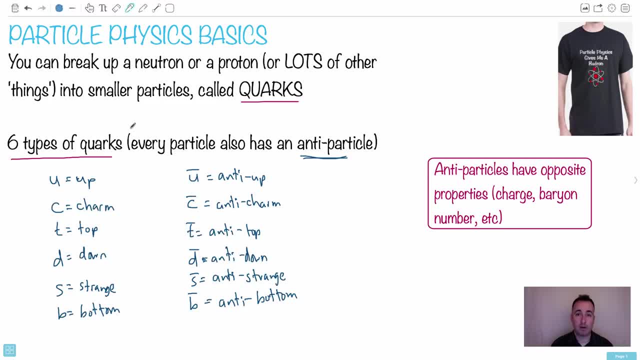 You know you can have. baryons are made of three quarks. Baryons are also hadrons. Mesons are made of two quarks, where one quark and an anti-quark, And those are also examples of hadrons. 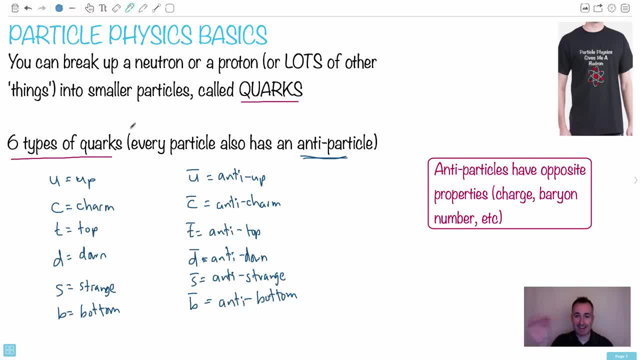 I think what I said, by the way, is all true, And yet I think if you write it all in sentence form it's not very clear. So I'm going to be repetitive to annoy you, But because I'm going to annoy you. 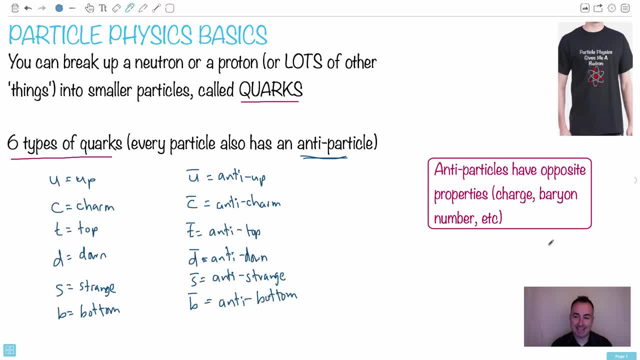 you're going to learn the structure really well, sort of how they're related. So this is going to sound slightly annoying. If I'm annoying you, good, I mean you know it. So what do we do with quarks? We have the 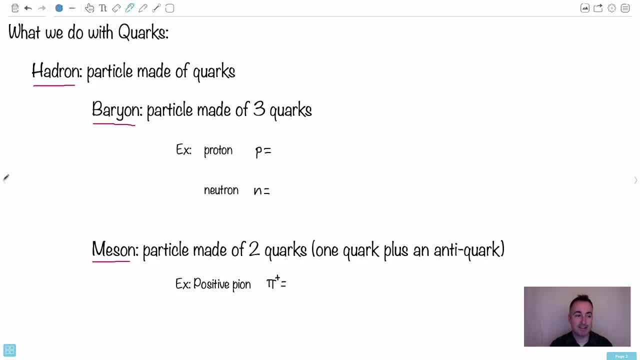 Largest scale structure with this is called a hadron. Or like this t-shirt, right, Particle physics gives me a ha ha ha. So what do we do with quarks? Hadron is a particle made of quark, So just think of that. 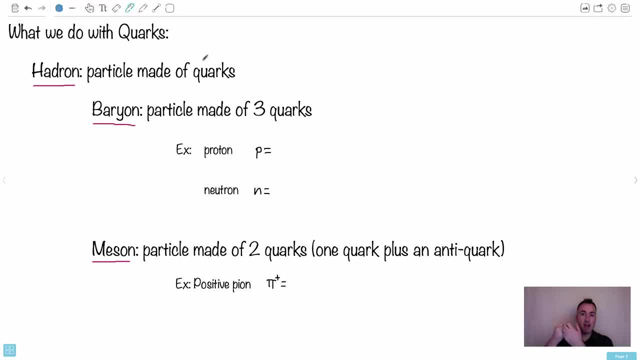 There's nothing else needed. You take some quarks and you make something out of it That's called a hadron. That's it. I like to think about hadrons as heavy, So there's like the heavier particles Now within hadrons. if you're going to make something out of quarks, 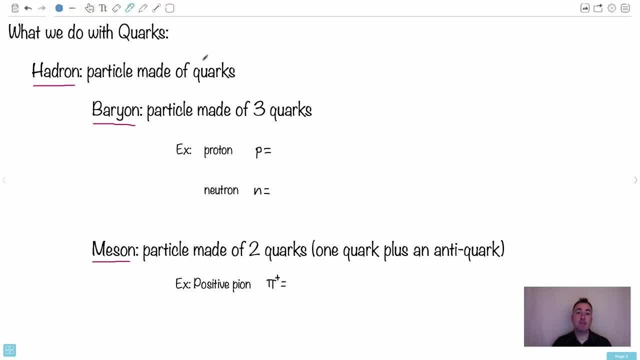 you can make two different types of particles. You can make something called a baryon, And that's when it's got three quarks. So again, baryons are just three quarks put together. You can have any of them. 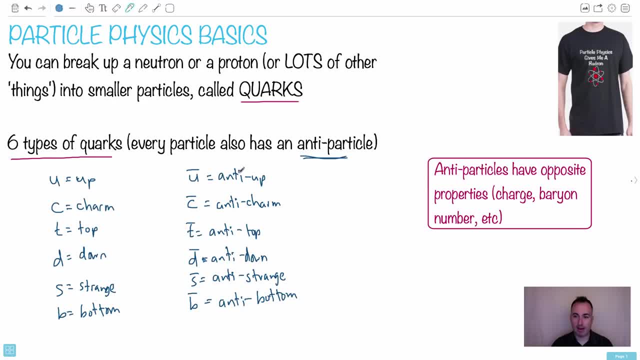 except obviously not an up, and it's anti-up because it's also, you know, annihilate. But as long as you have any quarks, any three quarks, or even anti-quarks, just choose three out of these 12, so long as there's never like a, you know. 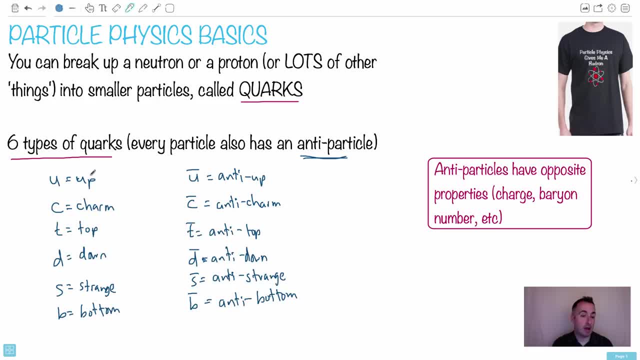 a quark and its own anti-quark. together You can have like an anti-top and an up and an anti-strange. I guess You'd have to check for conservation To see if it's possible you could check the Feynman diagram. 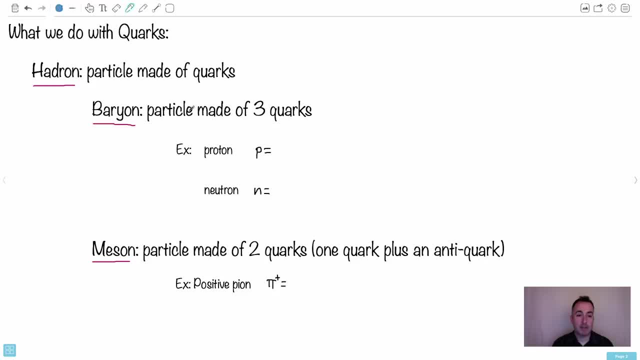 but if you can draw it, then it's possible. But if it's made of three quarks, we call it a baryon. That's it. So again, baryons made three quarks And of course, you made it out of quarks. 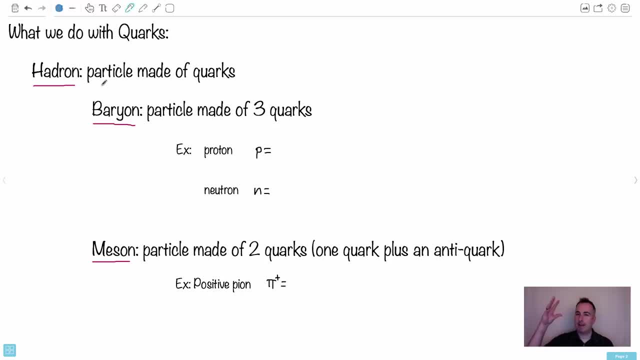 Therefore it's a hadron. So do you see the structure, Make something out of quarks called a hadron. If you make three quarks together, that's called a baryon, which is also a hadron because that's made of quarks. 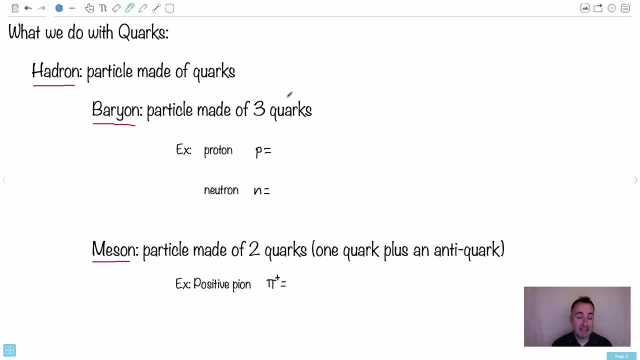 See repetitive. So there are two types of particles you need to sort of memorize, or at least know the structure, for You need to know the quark makeup of a proton. So proton is going to be made up of this, It's going to be up up down quark. 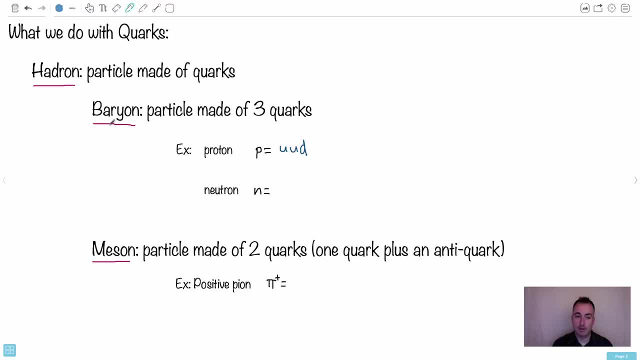 So it's got three quarks, right. See, three quarks. That's why it's a baryon And because it's made of quarks, it's a hadron. It goes up up down. Now does the order matter? 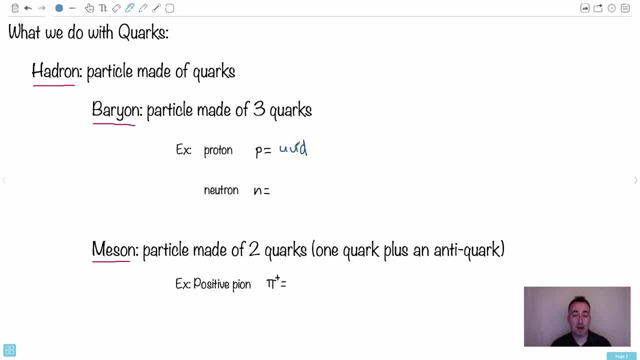 No, You could say it's down, up up. You can say it's up, down, up. It doesn't matter The fact that it has two ups and a down. that's the important part. A neutron, however. 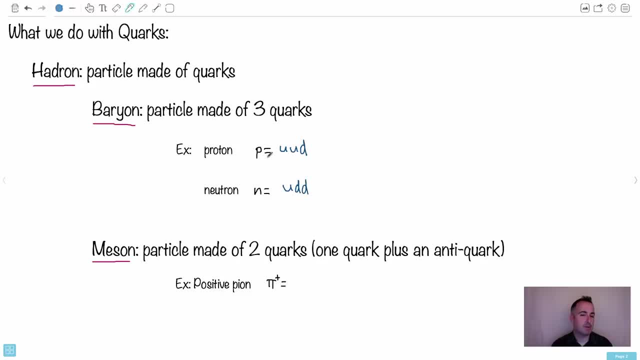 is up, down, down, So it's very similar to the proton right. It's only that there's a difference between one of the ups is a down. This is a little bit lame how I remember this. okay, Because you do need to know this. 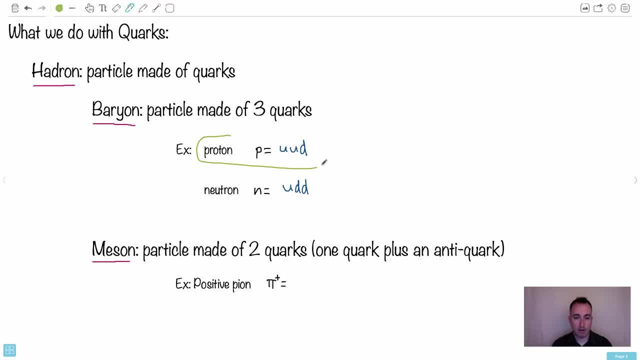 Okay, so I'm going to put this maybe in green here to circle it. So you do need to know this one And you do need to know this one. Those could be asked, It's implied at least. You'll need to know the makeup in order to continue. 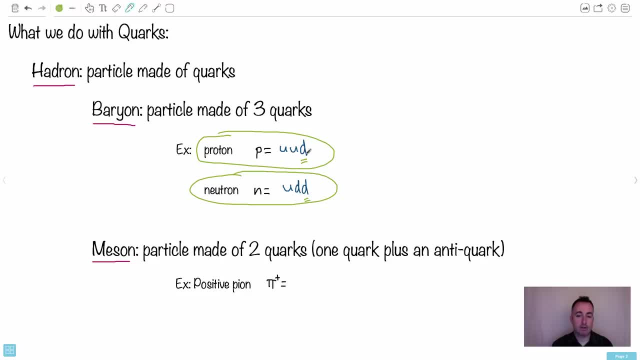 It's kind of lame, but I remember that both of them end in a down, So those are sort of the same, The way I remember the difference between a proton and neutron, I think like pro means, you know, we kind of use like the word, like positive. 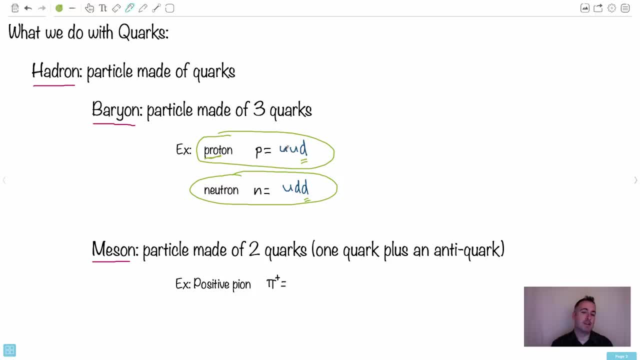 If you're positive about something, you're pro something. So look at this, You're up, up. It's almost like you know you're feeling like up, So you're very uplifted, So it's like you're very, very happy. 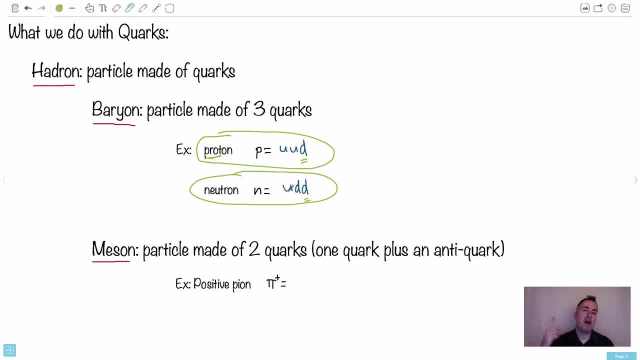 So that's why you're pro, Whereas a neutron, you're sort of neutral. Look, you're up, but you're also a little bit down. You're sort of you're in the middle, You're neutral. So I remember that the up down. 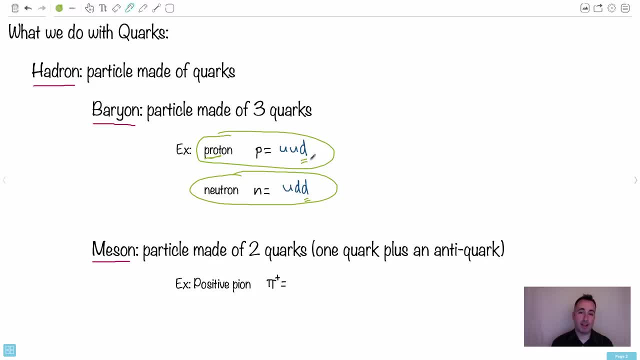 that makes me think of neutral. If that's really too lame for you, no problem, Just remember these and you're fine. Okay, so those are the two baryons you need to know about. And baryons: remember three quarks. 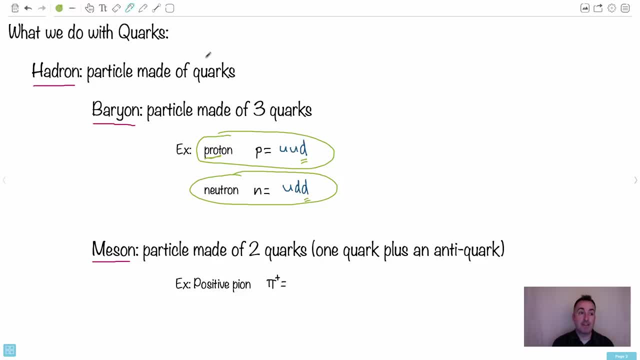 and you're also a hadron because you're made of quarks. There's another type of hadron, though. What if, instead of making three quarks together, you put in two quarks together, where one is a quark and one's an anti-quark? 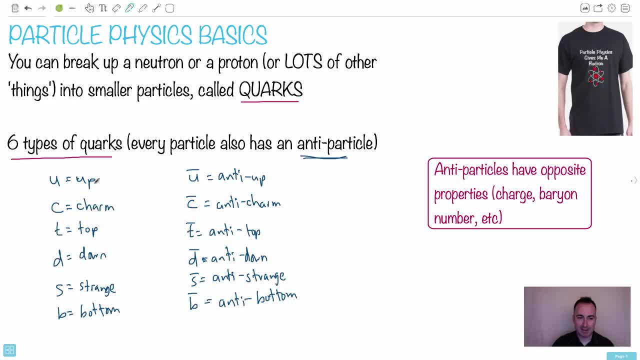 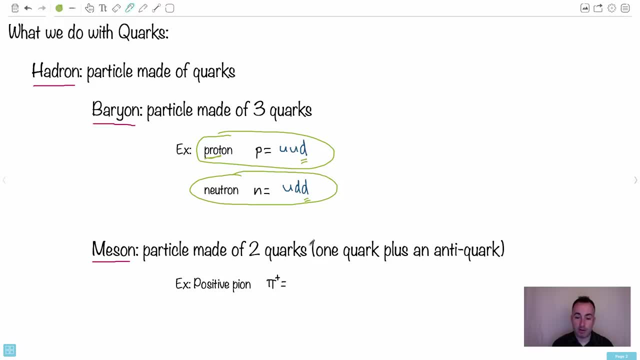 but not its own. Remember, because if you put a quark and it's anti-quark together, they disappear, they annihilate. So look at this, A meson. it's a particle made of two quarks, Like I said, a quark and an anti-quark. 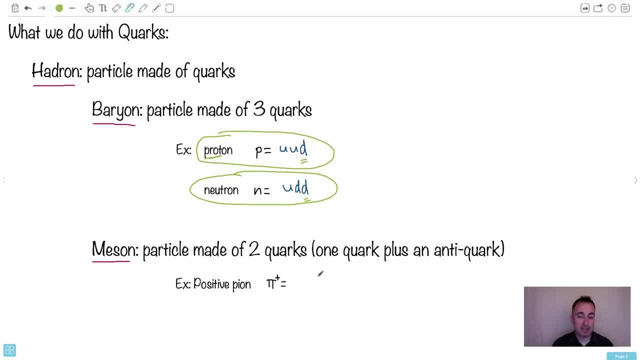 An example could be the positive pi. You don't have to memorize these ones. You'll. normally you'll be given the quark makeup of these things. But for example, there's one called a positive pion. That one, its quark makeup is: 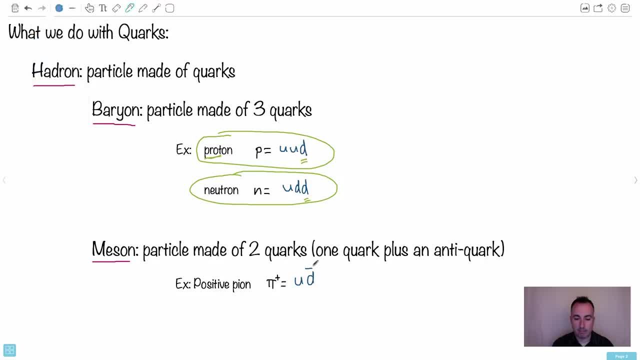 let's see here that would be up and anti-down. Do you see? There's only two quarks together, There is a particle and an anti-particle. So this is a meson, This is a real particle. You can actually find this in nature. 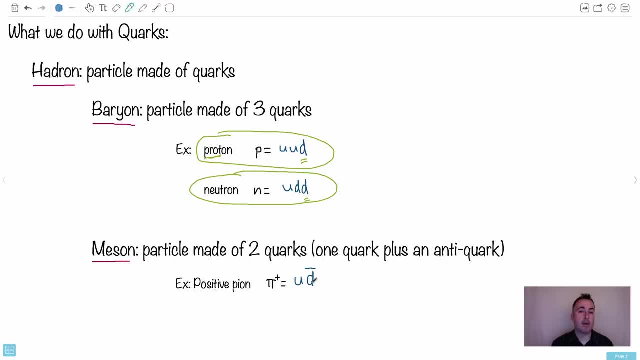 Some of them are very short-lived, for example, but this is a positive pion it's called, So this is really important. Again, remember: if it's made of a quark and an anti-quark, then it's a meson. 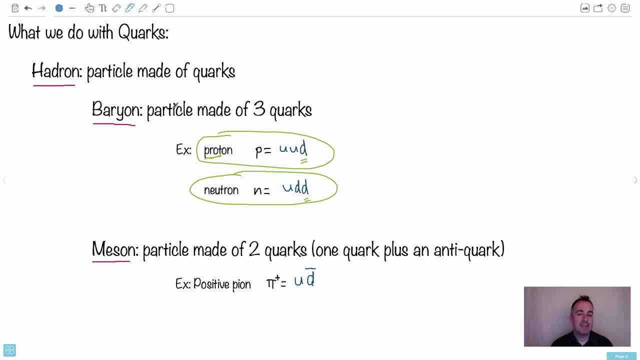 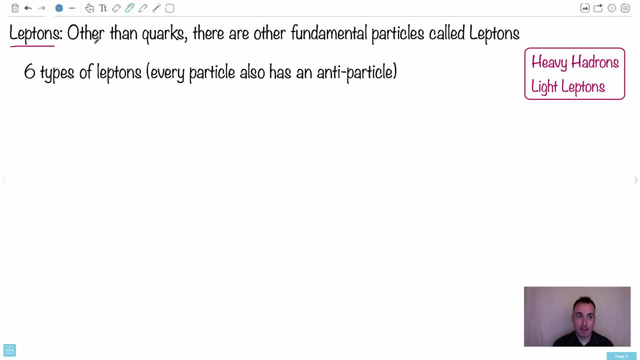 And remember, mesons are hadrons because they're still made of quarks. So this is how we could sort of break it all down here. So we've got other particles as well, called leptons. These are because, remember, we've got these basic fundamental particles. 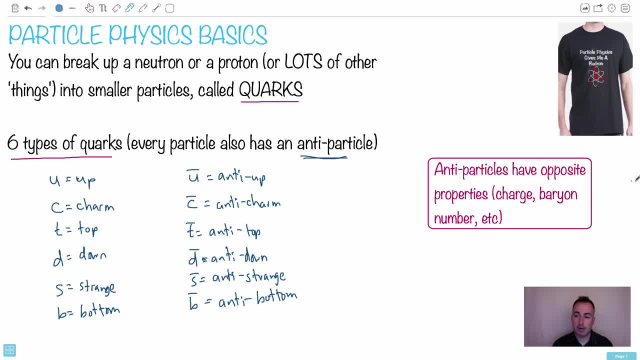 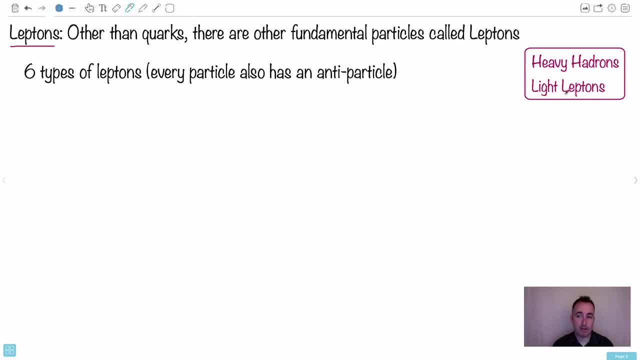 the light-based particles. the light-based particles, the lighter leptons, just like I think of the heavier hadrons. That's what I think about. So, lighter leptons and heavy hadrons. There are six types of leptons as well. 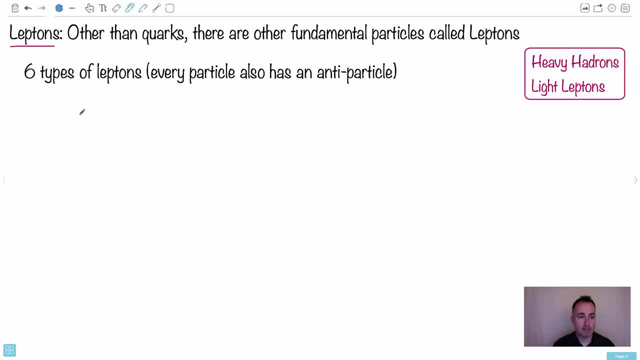 So let's put those down. These go as follows: There's one called tau. At least we call it tau. I heard it was one of my students. she's Greek. she told me they say it. I think they pronounce it taf in Greek. 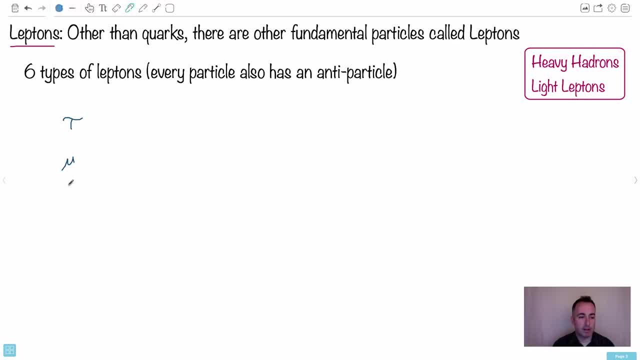 but I'm gonna call it tau. I'll ruin it. Then we have mu and then we have e, the electron. So this is the tau. By the way, these all have a negative charge. I'll put a little minus to the top right here. 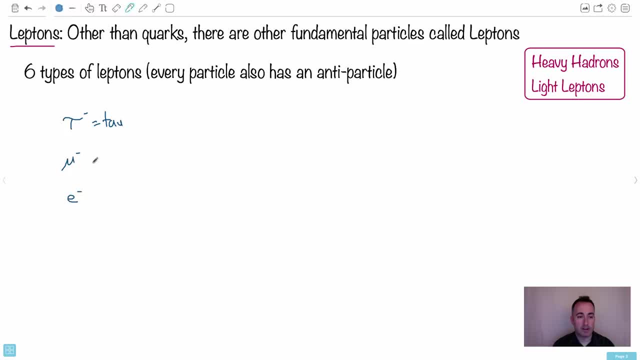 just to make sure we know. So this is called the tau, Some people call it the tauon. This is the mu particle. So some people call it the muon. This is the electron. Hey, that's a particle we know. 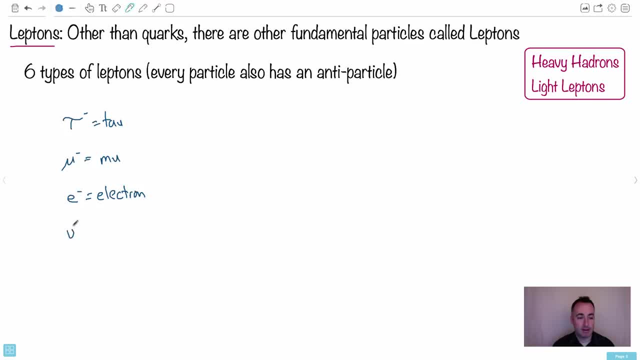 Then we've got something else Here. you've got these neutrinos. That's why we use the Greek symbol nu- Isn't that clever Neutrino. And we have these little subscript. We're gonna have three different neutrinos. 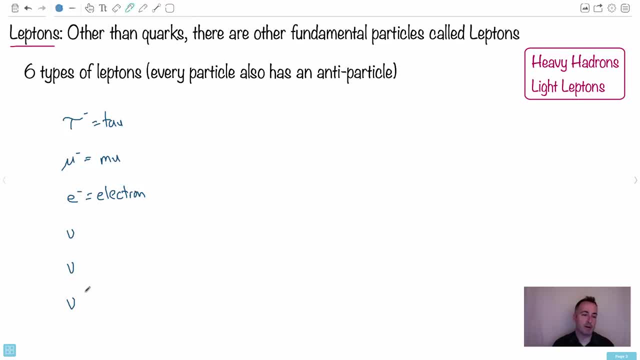 It looks like a V that's had one of its branches sort of blown away. It looks like a lot of wind has been blowing on this one instead of bending, So we put a little subscript. We have a subscript tau. We have a subscript mu. 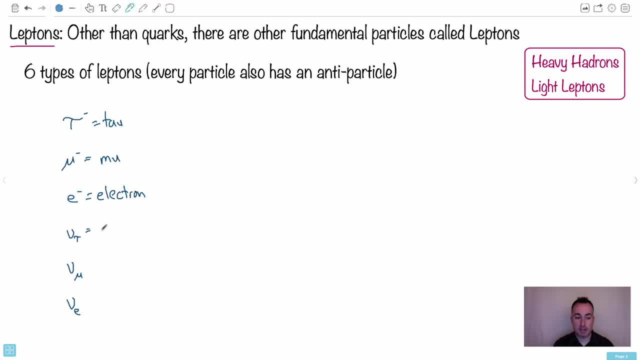 And we have a subscript, e Do you see, In other words, we call this the tau neutrino, That's what we call this one. We call this one here the mu Whoops. I should say the mu neutrino or the muon neutrino. 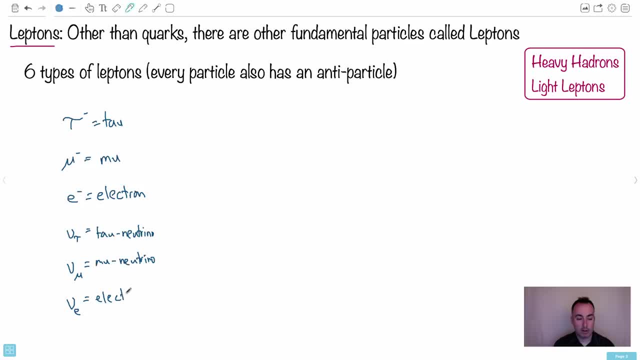 some people say: And this one here is the electron neutrino. Now of course we have the six antiparticles as well. So we have the anti-tau, the anti-mu, the anti-electron, We have the anti-tau neutrino. 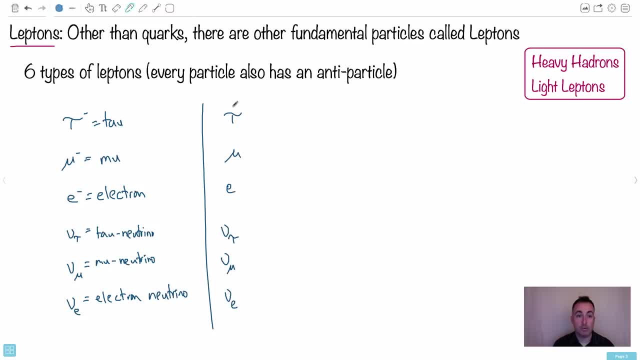 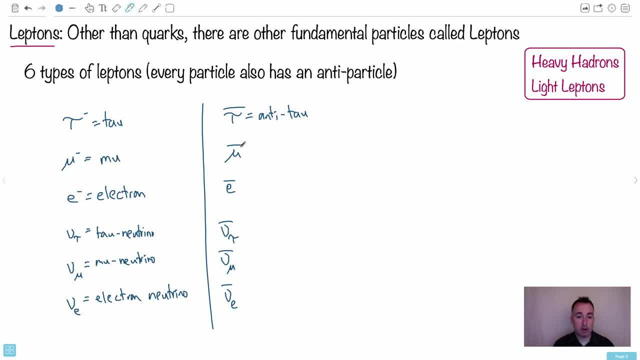 So I hope you understand this. Keep in mind, though, this particle right here- remember it has opposite charge, So if this had a negative charge, you could technically say this is. You could also write it like this, couldn't you? 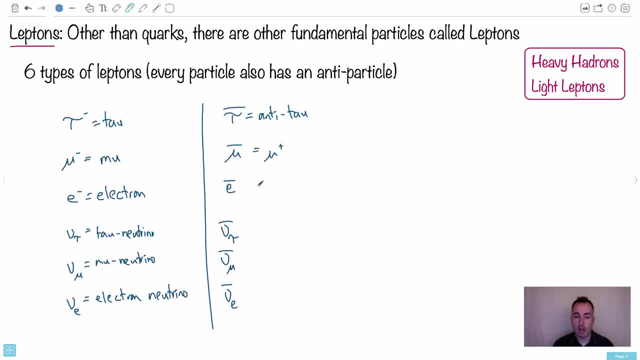 You could say it's a mu plus. That's also another way of writing this. Just like this: you could write it instead of the electron with a minus charge. you could also write it like this with a plus. By the way, this one has a special name. 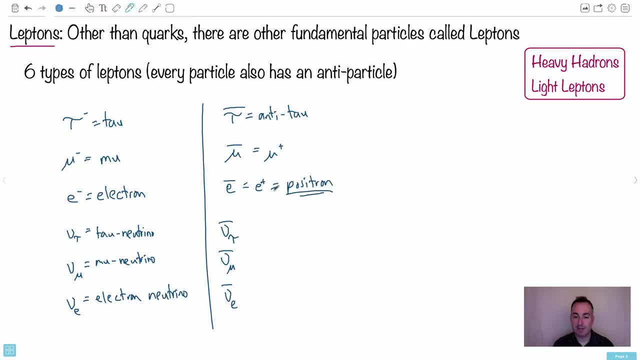 That's called the positron. So see, we have this electron and its positron, Those are the antiparticle pairs, And of course it's called the anti-tau neutrino, This is the anti-mu neutrino, And so on. 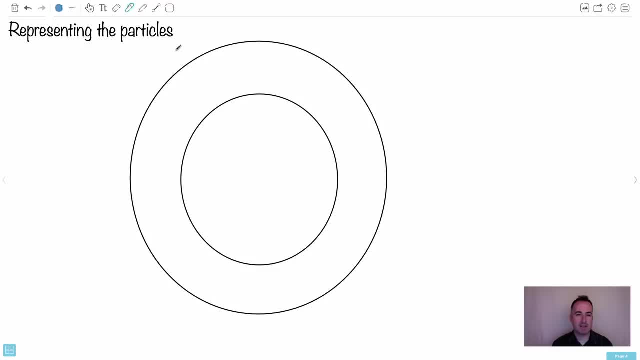 And very finally, then I think we have a nice way we can represent the particles. If we write sort of a line like this right here, then we can actually write them all down So we can say, for example, I like to put the u and c and t. 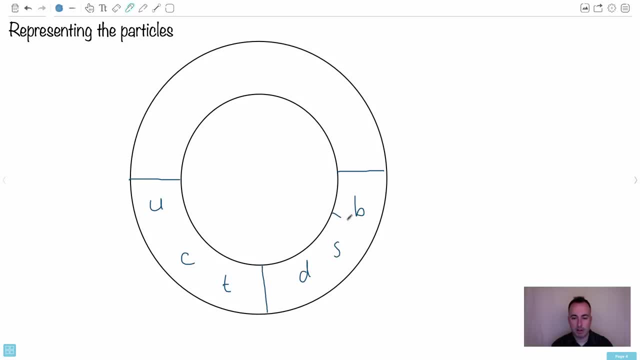 And we'll split them up and we'll put d s b. So these are all the different particles. we know This is like our zoo of particles here. These are the quarks, aren't they? So these right here, these are the quarks. 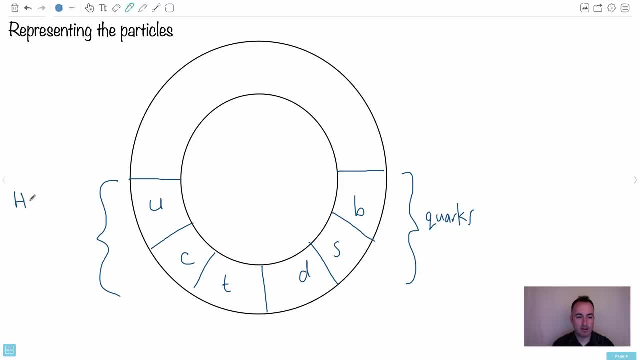 And remember if we put things together, if we make things out of them, these are called hadrons, Remember- I'm just trying to put everything together so we remember them, Hadrons, And remember what kind of hadrons we have. 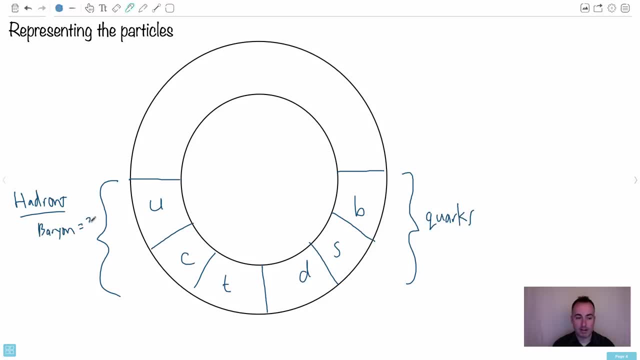 If we have a baryon, remember what that is: That's three quarks. And if we have a meson, remember that's two quarks, where one is a quark, one's an anti-quark And on the top, here we're going to have our instead of hadrons. 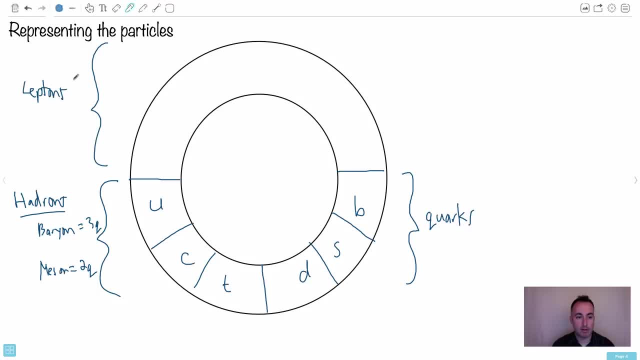 we're going to have our leptons. Those are the other basic particles, Remember. we can split those up and we can say, all right, we have the tau. And then we can split those up and we can say, all right, we have the tau. 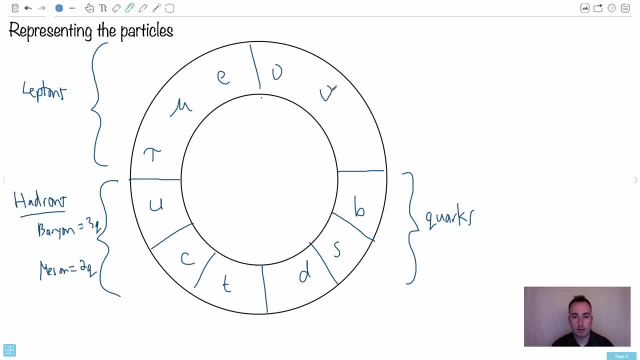 And then we can split those up and we can say: all right, we have the tau, Mu and electron, And then we have these three right here. These are the different neutrinos. I'm just putting them all down right here. 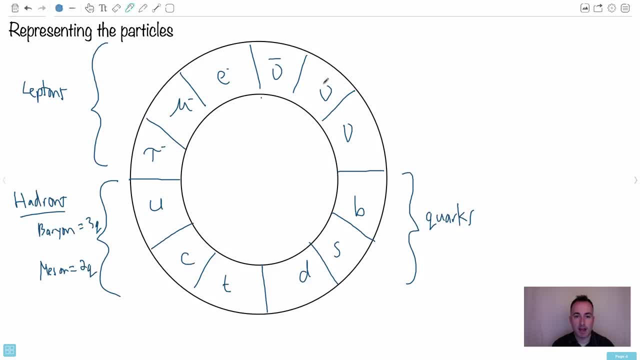 just so we can add up a little negative charges maybe on them, just like this. But these are the actual antiparticles here. These right here have a little tau and mu and electron. These are all our different particles. So this is it so far. 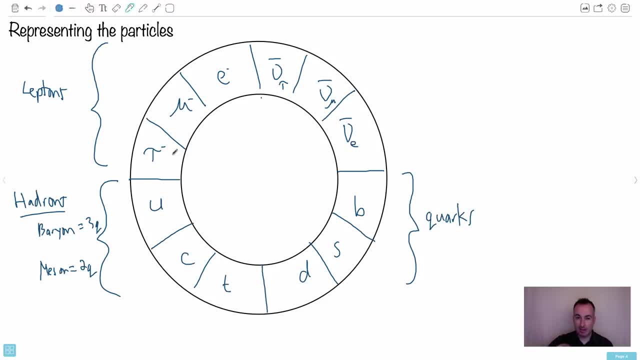 These are all the particles. I think it's a nice way to represent it this way. I actually saw this on a movie called Particle Fever and I really loved how they described it. I think it's a lot better than the ways a lot of other people show them. So that's why I use this.